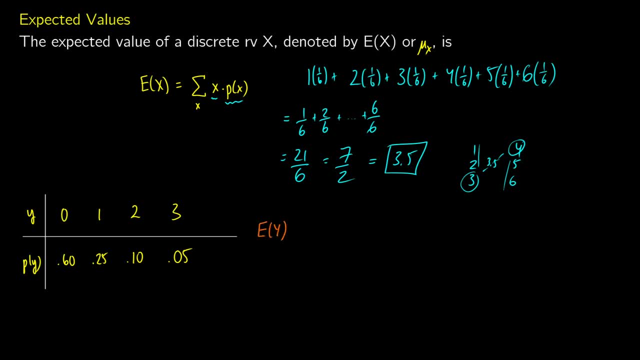 So what would be the expected value, Like how many times does the average person take the course? So what we can do is we can multiply each y value by its probability and we can add these together. So we get 0 times 0.6, plus 1 times 0.25, plus 2 times 0.10, plus 3 times 0.05,. 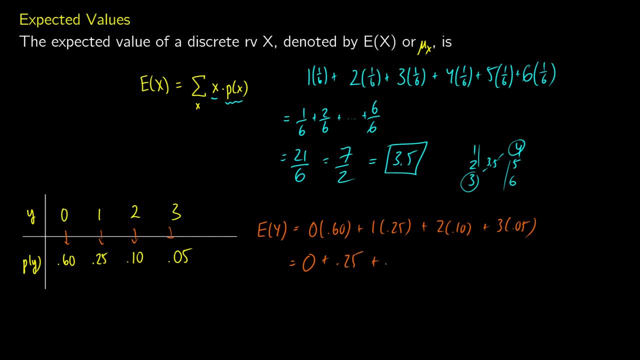 which is going to give us 0, plus 0.25, plus 0.20, plus 0.15.. We can add these all together and we're going to end up with 0.6.. So you could say, you know, if we were to pull, 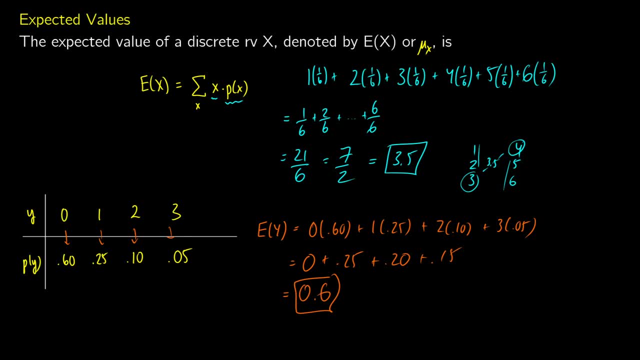 people infinitely, we would get an average of about 0.6 people end up taking the course, if that's what these y and py values represent. So that's how we can do it with just regular, discrete RVs using a table. So let's try another one of those. 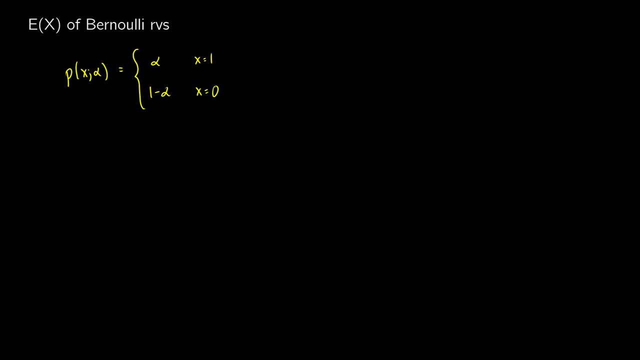 No, also think about Bernoulli RVs. So this is the case where you either have a success at a chance alpha or you have a failure. So how we can do this is very similar. If we were to draw a chart from this, let's just do our x and p of x here, the chance of it failing is going to be 1 minus. 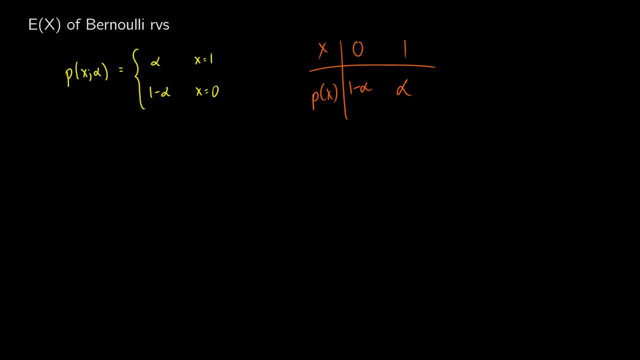 alpha and the chance of success is going to be alpha. So what this means to find the expected value, what we're going to do is we're going to take 0 times 1 minus alpha and add 1 times alpha. 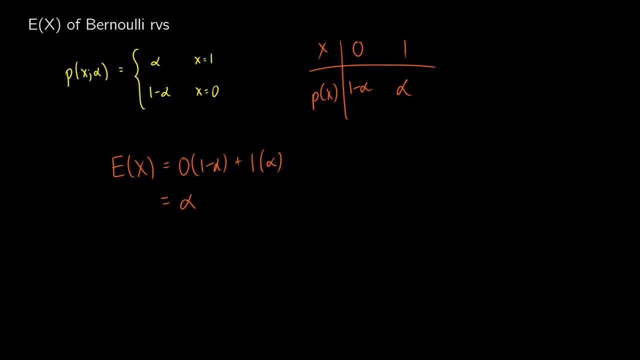 which is just going to give us alpha back when we multiply it out. So what this means is that the expected value of our PMF here is just going to be whatever. the chance of success is alpha. So let's say that we had some random variable where the chance of success is like 0.2.. 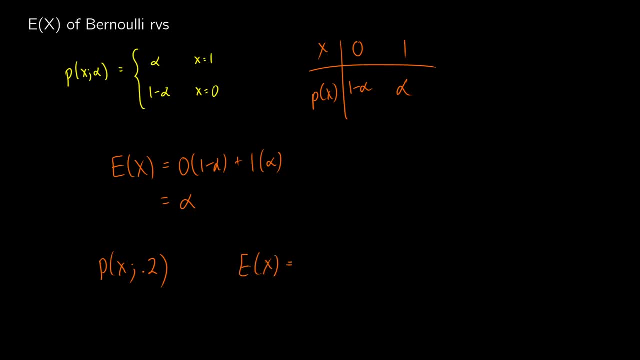 What's going to happen then is that the expected value is just going to be 0.2.. We see a success roughly 20% of the time. So let's take a look at a more complicated problem. Suppose the number of plants of a 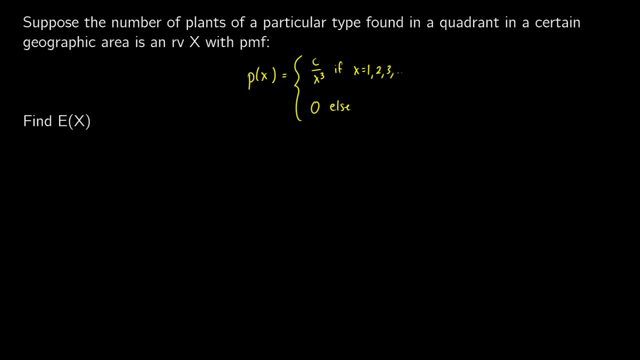 particular type found in a quadrant in a certain geographic area is a random variable, x, with the following PMF: It's c over x cubed if x is equal to 1,, 2,, 3,, 4, so on, and it's 0 otherwise. So to: 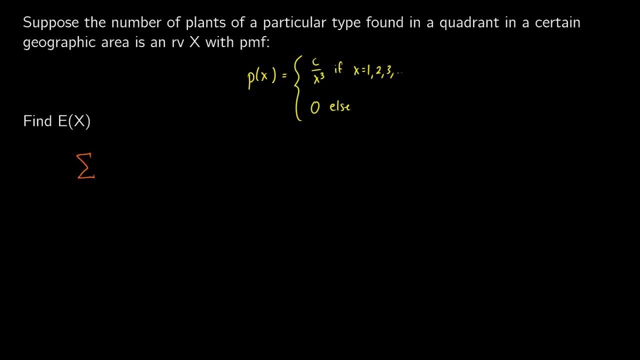 find the expected value. what we're going to do is we're going to sum all of our x's from 1 to infinity. we're going to take x times the probability of x. Now, this is going to be the same thing from x to infinity. x isn't going to change here. 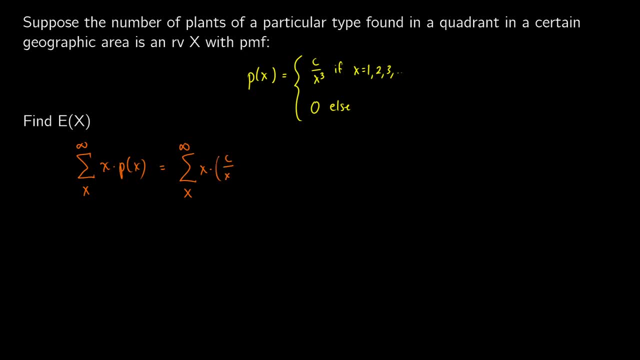 but we do know the probability at each point in x, which is going to be c over x cubed. Now, this is nice because we can cancel a little bit here. So we're going to get the sum from x equal to 0, which is going to give us x over x squared. Our probability of x is going to be another 10 frame per item. 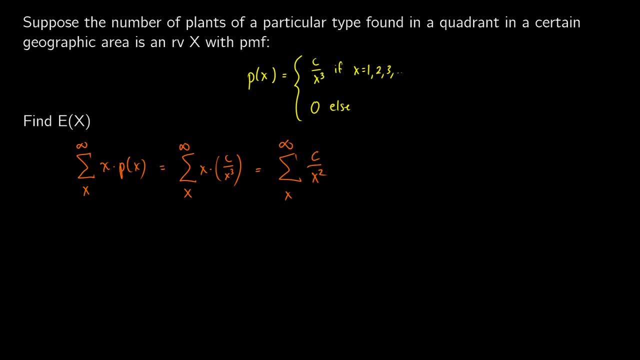 equals one to infinity of C over X squared. Now what do we know about this? Well, here we have our PMF. We're not gonna get a precise value because we have Cs here, but what we do know, maybe from calculus, is that if you take the sum of one to infinity, 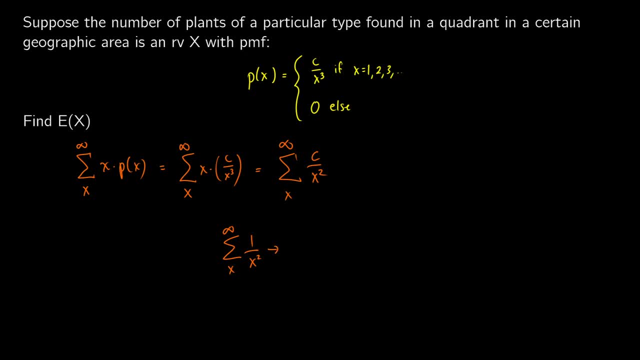 of X, of one over X. squared, this is going to 10, down to zero. So, although we might not know the specific value, what we do know is that it is finite. So we can get a number off of this, depending on what our C is here. 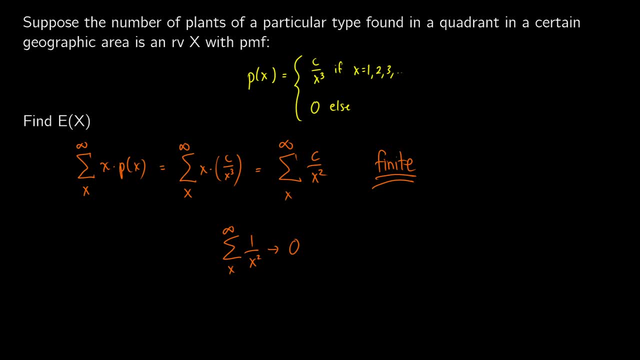 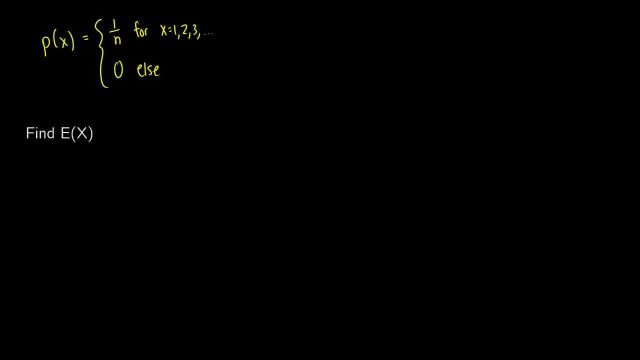 And we know that eventually, as we go on further and further, the probability is going to be very, very close to zero, as X gets very high. Now here's another one. Let's say that the probability of X is equal to one over N. 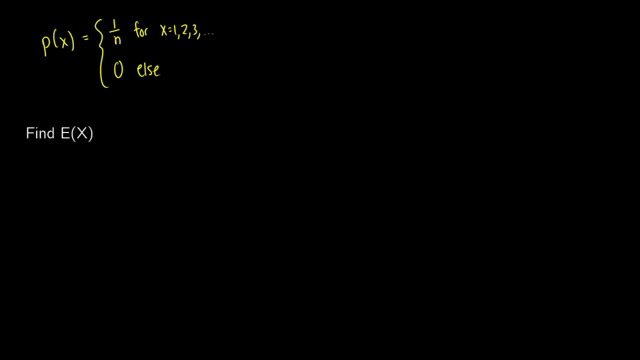 or X is equal to one, two, three and so on. So we know that the probability of X is equal to one over N and so on, and it's going to be zero else. So we're gonna do the same thing here. 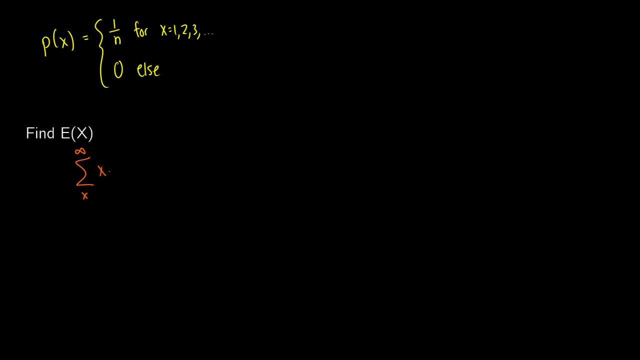 We're gonna take the sum, from X to infinity, of X times P of X, but here we know what our P of X is: It's going to be one over N. Now this looks like something that we can do a little bit more with. 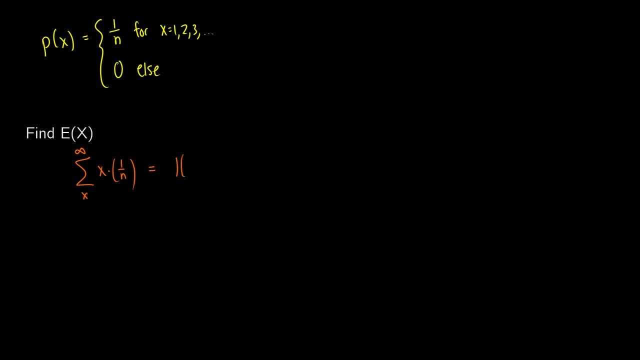 because if we plug in values for X, this is going to be one times one over N, plus two times one over N, One over N plus three times one over N, plus so on. So, using this fact, perhaps we can get a little bit more clever with it.